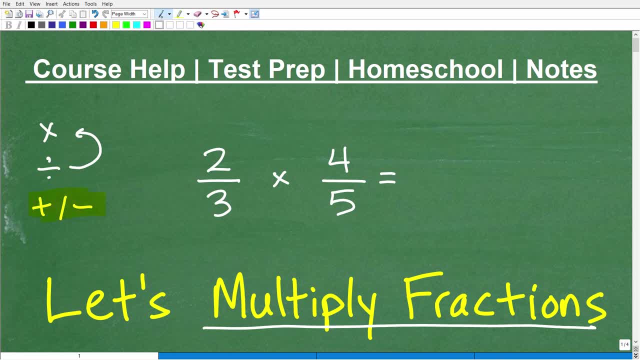 With fractions. these are a little bit more involved. so if you are struggling in any of this stuff, I'm going to give you some suggestions as we go through this video. But here is a basic problem, and if you want to go ahead and pause the video, just quickly think about: hey, can I do this? Do I remember how to do this? We all learned how to multiply fractions. but the idea is: do you remember? Okay, so we're going to get to all this in just one second, but first let me quickly introduce myself. My name is John. I'm the founder of TabletClientcom. 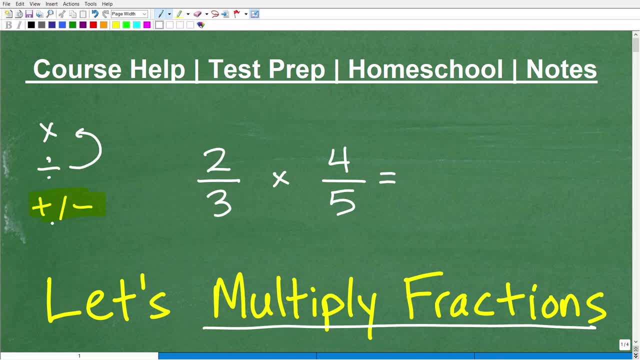 I'm also a middle and high school math teacher. I'm going to leave a link to my math help program in the description of this video. But if you are one of these people that really don't think they're good in math, maybe your self-image of yourself is: I've just been bad at math for years. I failed math, so therefore I must be bad at math and I need to steer clear of it. Or maybe you're frustrated in math currently because, whatever reason, maybe you're not good at math. 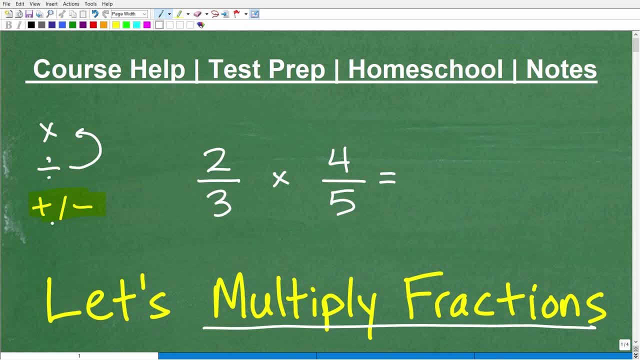 Maybe you're not getting enough math instruction or maybe you're not connecting with their teachers teaching style. I'm just here to tell you: everyone can be successful in math. So even if you haven't done well in the past, I can help you out Now. I've been teaching math for decades and my approach to math is a little bit different, because I really work on students mindsets and I'm here to tell you one: if you have the desire and you're willing to work towards learning mathematics, that can help you out. I really break things down in a clear and understandable manner. So if you're at the middle school, high school, 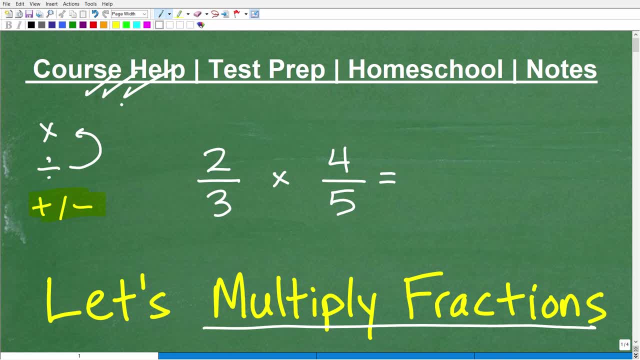 or even college level in mathematics, you definitely want to check out my math program to help you out. Now, if you're preparing for any test that has a math section on it- I'm talking about things like the GED, SAT, ACT, GRE, GMAT, ASVAB, ACCUPLACE or CLEP exam, teacher certification exam- you get the idea. I have excellent test prep courses that can help you prepare and pass those exams. If you homeschool, you definitely got to check out my comprehensive homeschool math courses and curriculum. And if you don't have any math 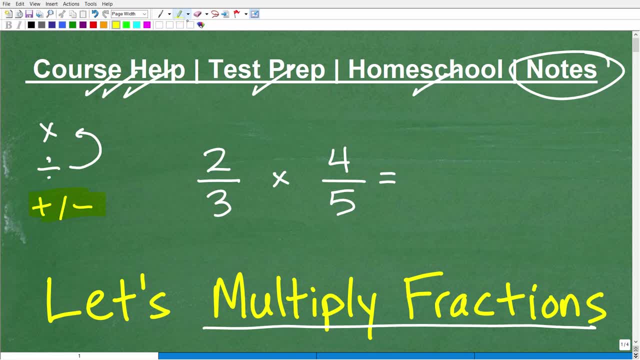 notes. I'm going to leave links to my math notes. If you want great grades in mathematics, you must learn how to take great math notes. So start improving your notes and you'll see your grades increase right along. All right, so let's take a look at this problem. two thirds, excuse me times. 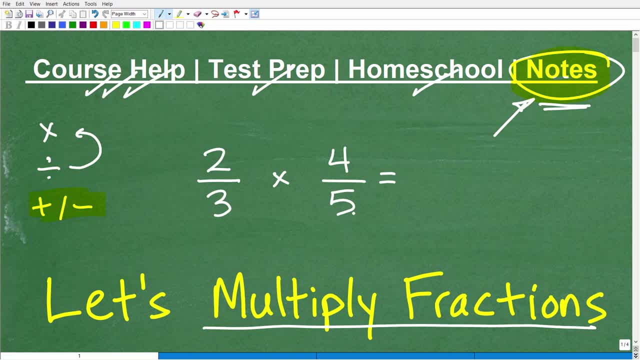 four, fifths. Now, one thing you do not want to do. right, some of you are like fractions- this might be your expression. you know it'd be like: oh, I don't want to deal with fractions, why can't we just deal with nice easy numbers? well, fractions are pretty common. you know forms of numbers and 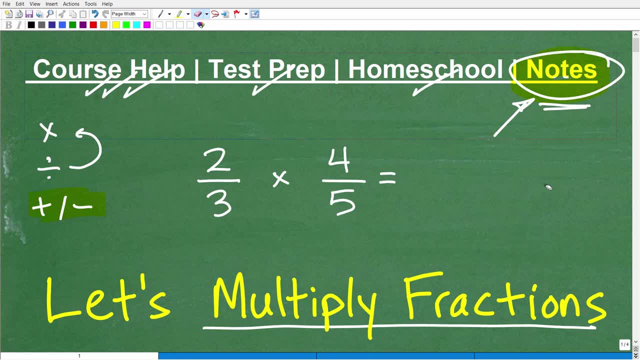 we're going to have to deal with them. One thing that you don't want to do, okay, is be like so afraid of fractions that you go into your calculator and you turn this into a decimal. you go, oh, two divided by three, you get that decimal. and you go four divided by five, you get that decimal. then you 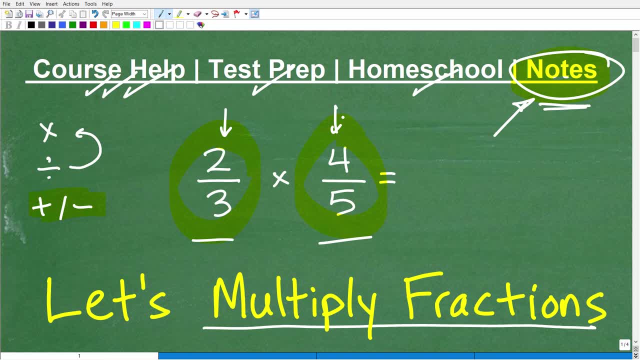 use your calculator as some sort of you know workaround. Now you put that calculator away because oftentimes you know what I'm going to be teaching here applies to algebraic situations, in other words, like a over b times, c over d. of course you can't put this into your calculator and get. 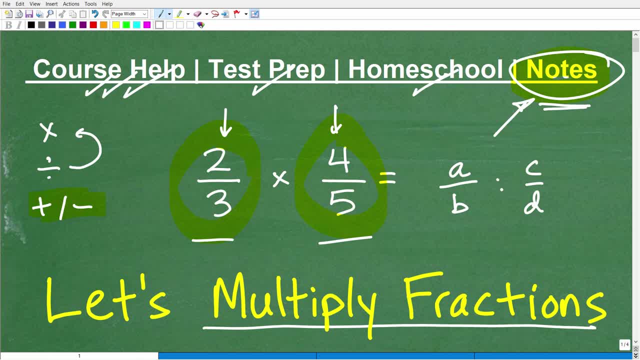 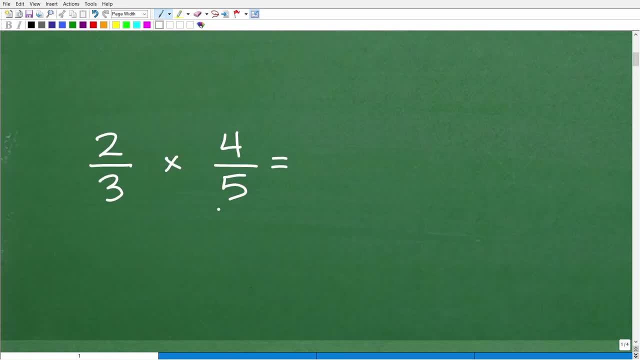 decimal equivalents, right, so we just need to know how to multiply fractions, and it's not that difficult. so let's get right to it. and again, if you know the answer to this question right, two thirds times, four fifths, put that into the comment section, because I'm going to answer it right now. 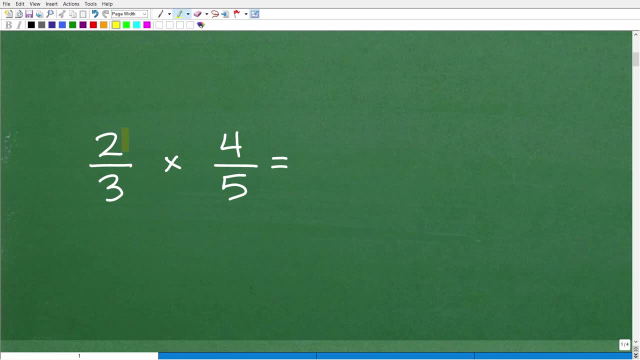 Okay, so what do we do here? well, let's just get some basic definitions down. when we're talking about fractions, the top number is called the numerator and the bottom number is called the denominator. okay, so in this particular fraction, two is a numerator, three is the denominator over. 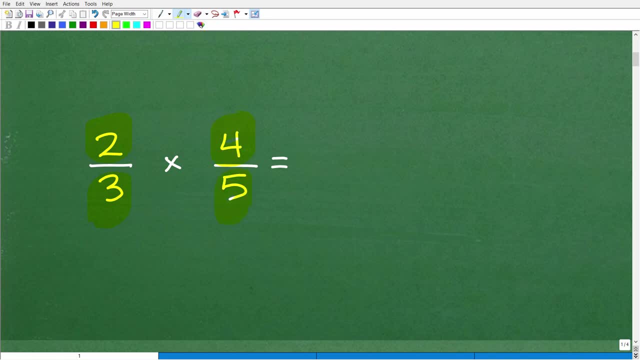 here, four is the numerator and five is the denominator. so the way we multiply fractions is we simply- let me just do this a little bit better- we simply multiply the respective numerators, okay, and the respective denominator. so in this case, we're going to multiply two and four, so that'll be. 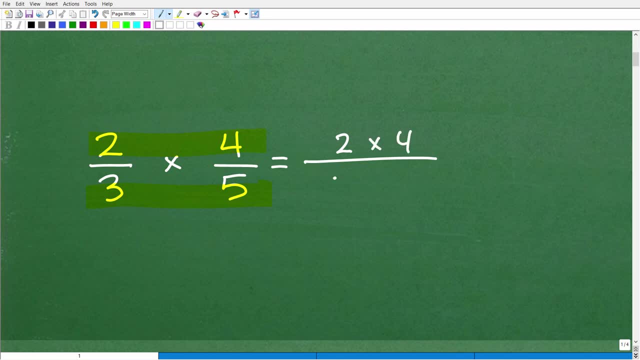 two times four over three times five. okay, so you can see, here I'll multiply the numerators over the denominators, and when I do this I'm going to get my answer. so two times four is a course eight, and then we have: three times five is fifteen and that is the final answer. now let's just talk real quick. 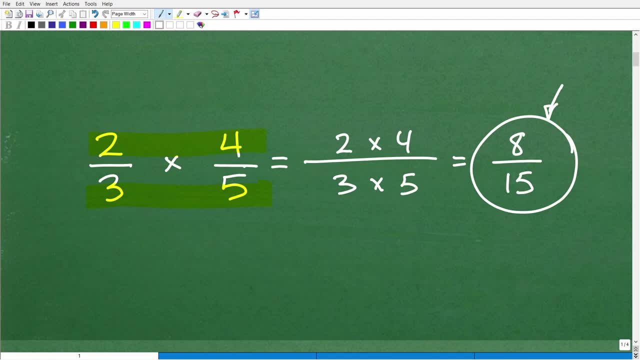 about the results. So here's the result of multiplying two fractions. okay, when you're doing this, you always want to end up with your most simplified, reduced fractions, so that's really, really important. so we'll do a couple practice problems here and I'll talk about, you know, how we can kind of do this as we work the problem. but you know, right now let's just make sure we understand how to multiply fractions. okay, just multiply the respective numerators and denominators and simplify and reduce and you are done. 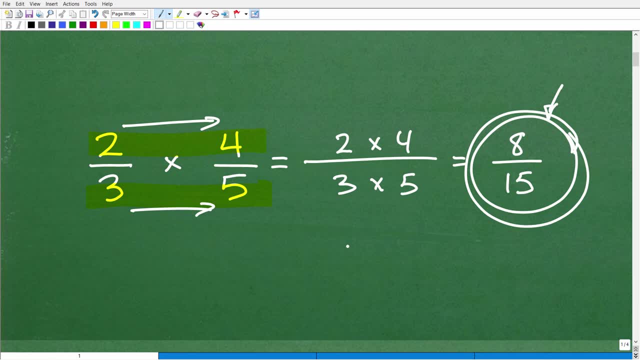 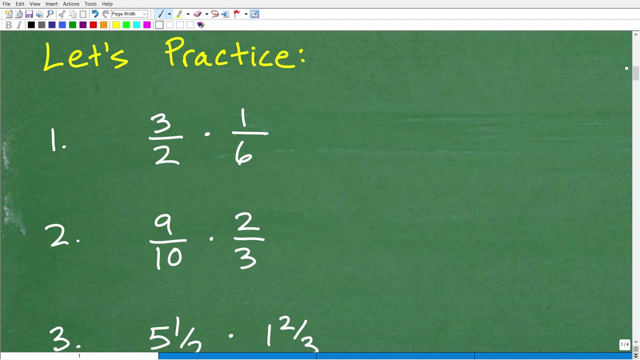 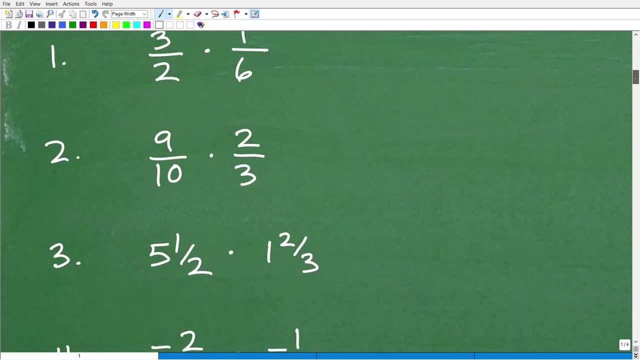 If you remember this and got this answer right without being lucky, well then I must go ahead and give you a nice little happy face and an A plus and a 100% for this particular problem. All right, let's move on to some practice problems now. all right, we'll just do these one step at a time. we'll do problems one and two. you could say I have problems three. actually, let me just show you problems one, two and three. I have one more down here. we'll leave that here for a second. so 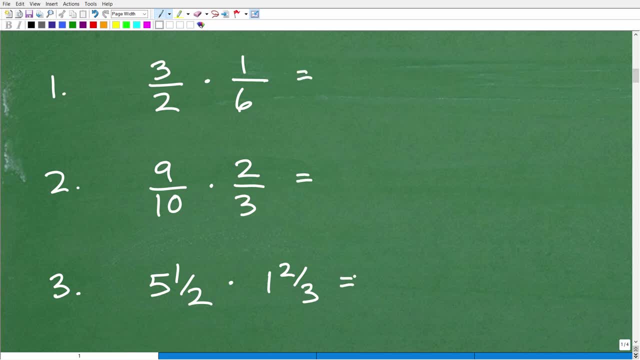 If you want to Excuse me, boy, my, my voice was crackling up there. maybe it's because all these videos I've been doing lately, but anyways, that's not gonna let me stop the video. let's proceed. so here we have three practice problems: three halves times one, six, nine, tenths times two thirds, and then five and a half times one and two thirds. go ahead and pause the video, get a piece of paper out, a pencil, and knock out. these problems are real quick. this is the best use of this video. if you're watching this video and you really want to. 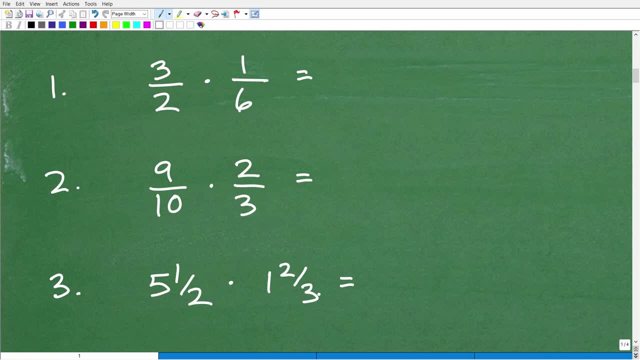 You know, understand how to multiply fractions. it's not enough just to watch me do a problem. be like: okay, now I know, now you got to practice this stuff, so let's go ahead and practice this. and of course, number three has a little bit of a twist to it. we'll talk about that here in a second. 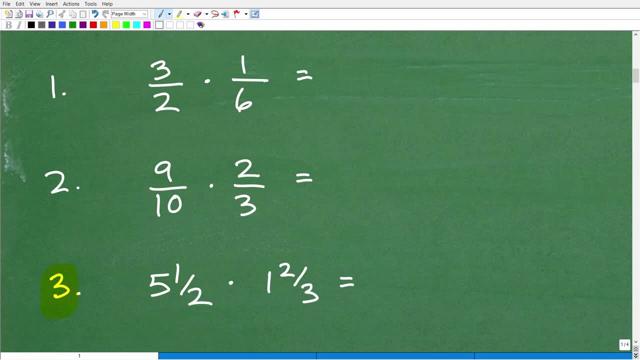 Okay, so hopefully you pause the video and did these problems. let's get right to it. so we have three halves times one, six. so what do we do? well, here We have our, these fractions, what we call Improper. this one's called an improper fraction and this one's called a proper fraction of. basically, what you need to know is that we only have one numerator and one denominator, one numerator and one denominator. so the result again, we're going to multiply the respective numerators and denominators, so it's gonna be three times one over two times six. of course, that's going to be three over twelve. now, looking at three over twelve, my question to you is: cannot be reduced? okay, yes, it can be. three goes into twelve. how many times? 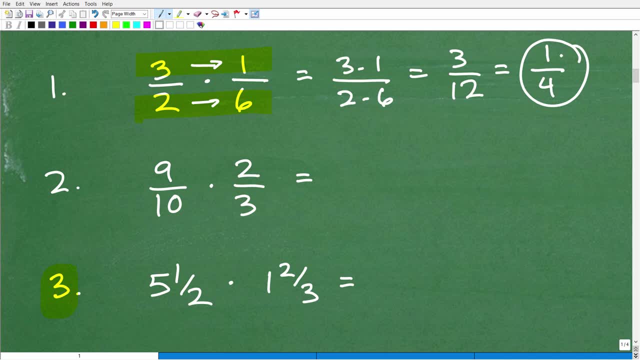 Okay, four, so this is one fourth. this is the final answer. okay, so we got that very good. now let's take a look at how you could do this kind of cross cancel some factors. so some of you out there might be like, okay, three goes into six, two times. okay, this will probably- you'll probably remember this one school. and then you're like: okay, that's one over two times two, which is one fourth. all right, so you can kind of cross cancel factors. but I didn't want to 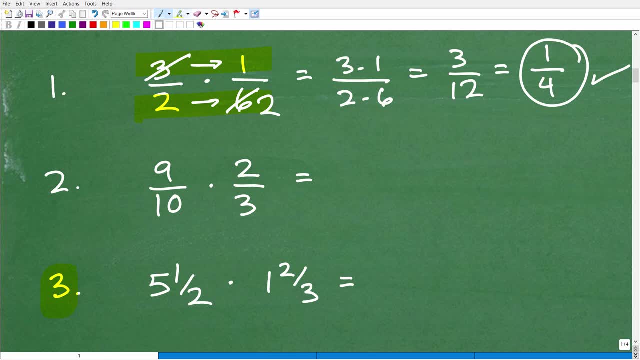 Okay, introduce that because we want you to really make sure you just understand how to multiply fractions, and then you can just deal with this fraction and reduce it to its final form. okay, but if you're comfortable across canceling factors, go ahead and do so. so let's take a look at this problem. we have nine tenths times two thirds. so again, we're going to multiply the respective numerators and denominators. so nine times two is, of course, eighteen, and then ten times three is 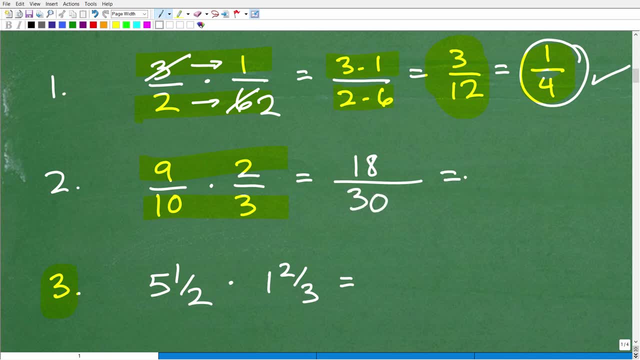 thirty. Now I can reduce this and this is reducible. but let's take a look at our factors here. okay? so Let's say: okay, three here goes into nine. how many times? these are factors? this is being separated by multiplication. so three goes into nine: three and two goes to ten five. okay, so two goes into ten five. so is our answer: three fifths. it is, but let's, let's work on that real quick. I'm going to put 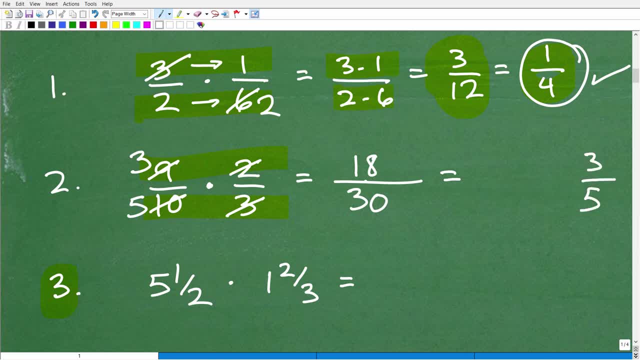 Put this over here and let's just look at how we reduce this fraction here. so you'll look at eighteen and thirty and think about this for a couple- you know some seconds here- but like okay, what number goes into eighteen and thirty? you're like: two goes into this, three goes into this, all six goes into both. okay, so six goes into eighteen three times and then six goes into thirty five times. so that's a separate discussion on how to reduce. 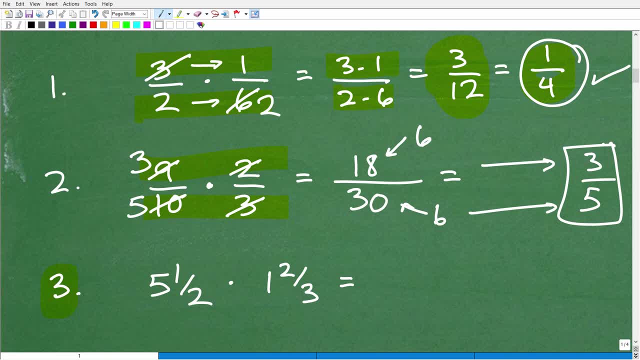 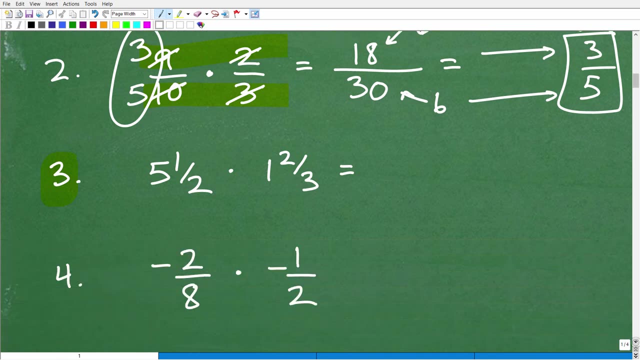 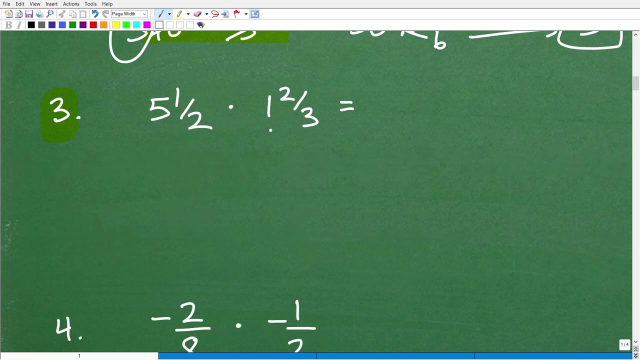 Fractions. but you definitely need to know how to simplify and reduce fractions by cross canceling, like factors. but you can see here if, if you're good enough at it, you could just cross cancel all the factors and get your final answer right there. okay, so let's move on to this third problem and we'll deal with this fourth problem here in a second. so how do we multiply mixed number fractions? okay, so we have five and one half times one and two thirds. well, what we're going to need to do 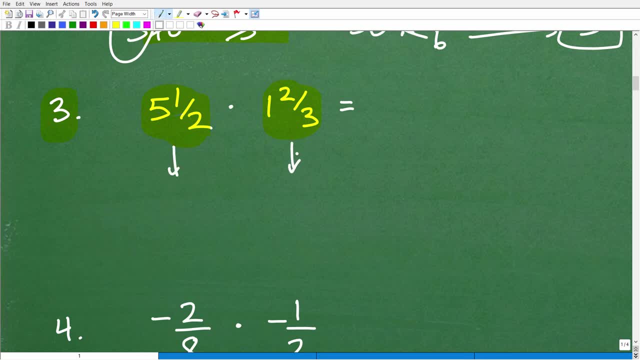 Is to convert these mixed number fractions into improper fractions. okay, so how do I do that? well, if you recall, we're going to take this little denominator right here, with this one half. we're going to multiply it by five, so that's two times five, which is ten, and then we're going to add one. all right, so two times five is ten, ten plus one is eleven, and then we put it over this denominator right here. so I'm going to be doing a separate video, and I've done many videos on how to. 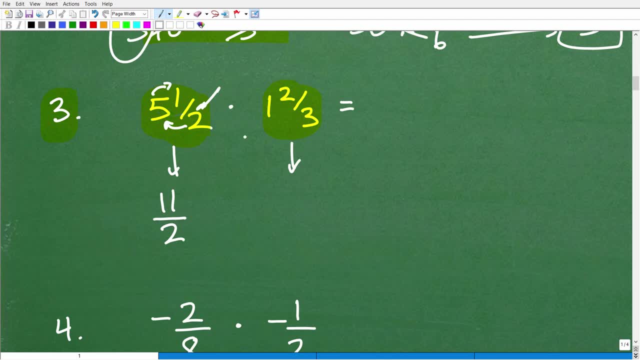 Change a mixed number fractions to improper fractions, but most you probably remember that. let's go ahead and do the same thing with this fraction. so three times one is three plus two is five. okay, so that's going to be five over three. now let's take a look at our problem here. okay, can we do any cross canceling of factors? this three going to eleven, this three going to five? nope, three does not go into eleven. does two going to five? nope, so none of this. 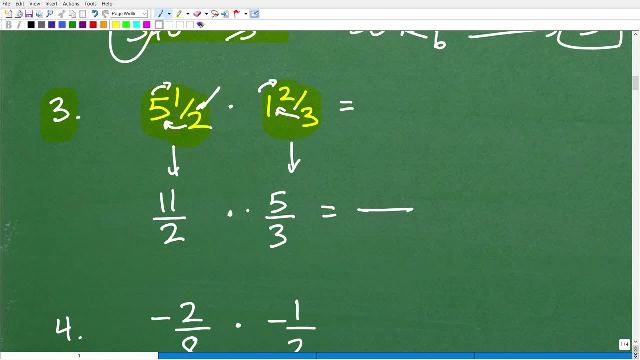 None of these factors can cross cancel. so when we do our final product here, okay, remember going to multiply the respective numerators and denominators. we're not going to be able to reduce, okay, so eleven times five, of course, is fifty five, and then two times three is six, and that is your final answer. now, here's the one thing that you don't want to do. now, a lot of you are going to feel compelled to take this improper fraction and turn it into a mixed number, in other words, 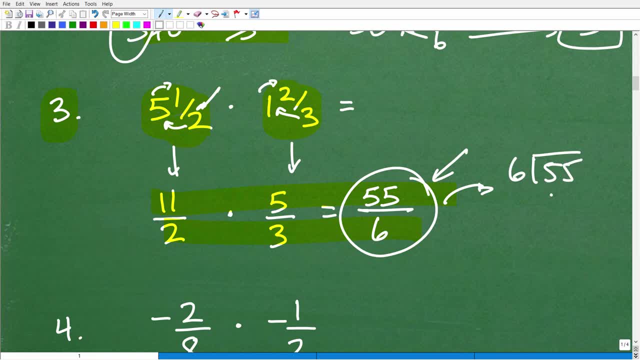 You're going to go- six goes into fifty five and you're going to start working this out. okay, do not do this. don't turn this into a mixed number fraction like this kind of voluntarily. now, if your teacher asks you to do that, then go ahead and do so. or if you need to do that because you need to recognize it on some sort of test, do that. but the main idea is, when you do this- I've seen this thousands of times- where a student will have the right answer, they'll go to. 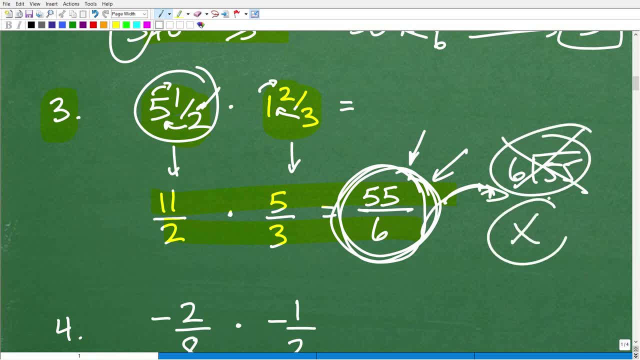 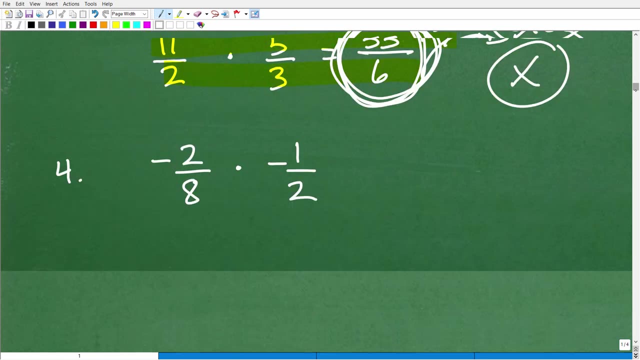 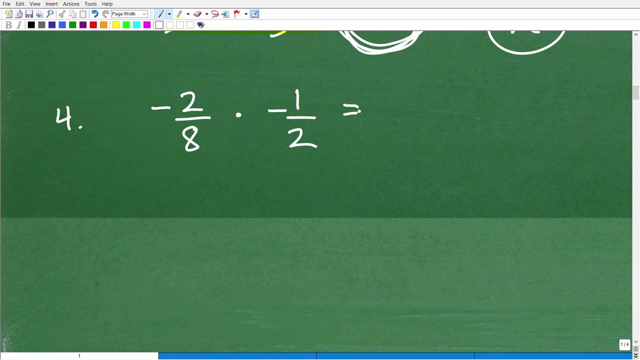 Convert this into a mixed number fraction and make a mistake. and then they deliver to the teacher the wrong answer. well, in fact, they had the right result. so just make sure your answer is fully simplified and you'll be good to go all right. so we got that right, then. that's excellent as well. and now let's go ahead and throw an additional twist to multiplying fractions, and that is if we introduce positive and negative number values. so as you progress, I don't know what level you're at. maybe you're at the 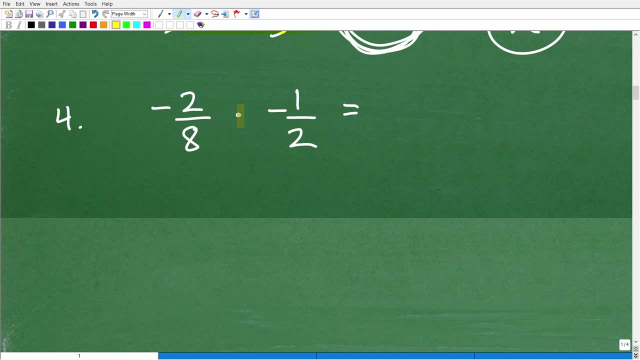 More of the basic elementary level math. but as you go into middle school and high school especially, you're going to be dealing with positive and negative numbers, but the rules don't really change. what we do have to do is just keep in mind what is going to be the sign of our answer. so this is multiplication. 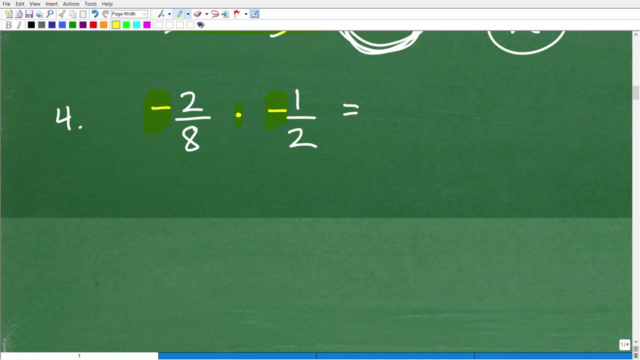 And we're multiplying a negative number times a negative number. so what is that? well, a negative times a negative is going to be positive. so once you recognize this is going to be a positive result, Then Just kind of don't worry about the signs, okay, just go ahead and work on the actual problem itself. so let's go ahead and do it both ways. we'll go two times one, which of course is two. eight times two is sixteen, and I can reduce this as one eighth. so that is the final answer: positive, one, eighth, or I can. 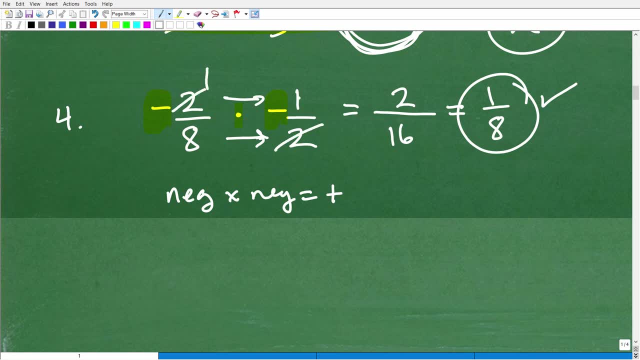 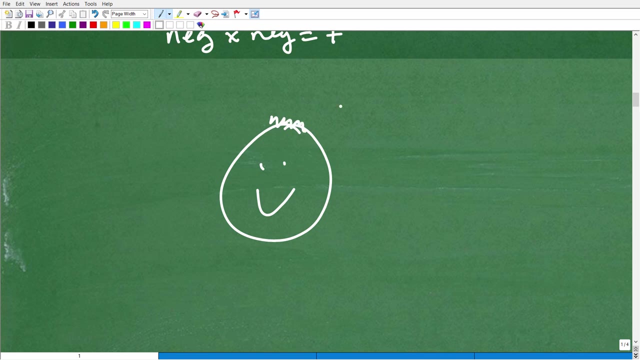 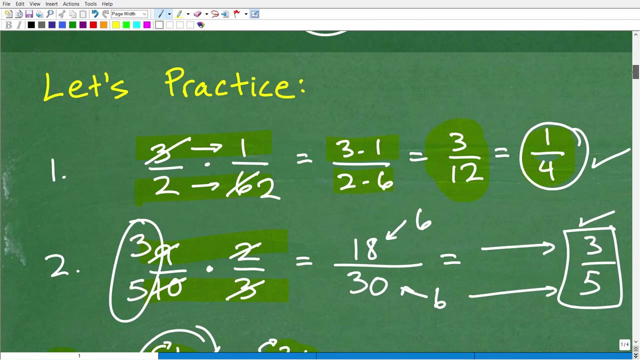 Go ahead and cross cancel these factors. two goes in this two, one and I'll live with one over eight. again one eighth, positive one eighth is The final answer. okay, if you got all these right, you're like, yeah, this video was easy for me. well then, listen, I must go ahead and give you a good old nineteen, eighty four flat top haircut with an, a plus and a few stars to make you feel extra special today. nice job, okay. now I would say these are pretty introductory level type of problems, but multiplying fractions, as you can see here, is pretty easy. okay, what is? 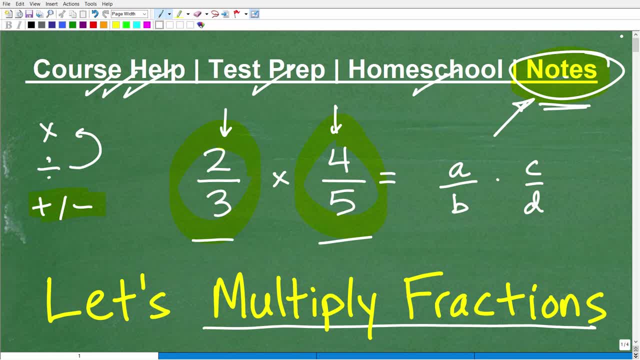 Difficult For students is remembering not to confuse multiplication with division. you know addition and subtraction and the only way you're going to be able to remember this stuff is through practice. but you want to practice the right way. okay, watching math, watching me do math- is not the same as you practicing problems. so if you don't practice and follow through, well, this is going to you remember this for maybe, like you know, thirty minutes and then it's going to go away. but anyways, hopefully, this little video. 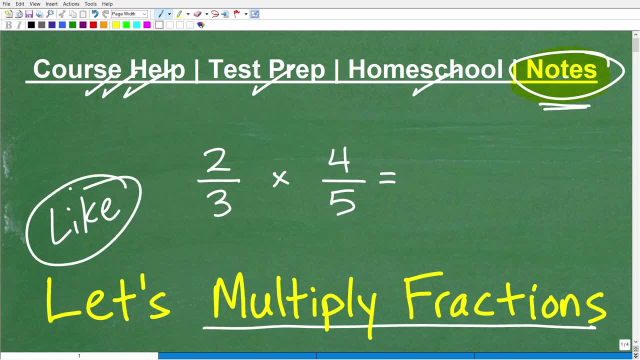 Helps you out. and if that is the case, go ahead and consider smash that like button. and I told you I was going to give you some suggestions on other fraction topics like addition, subtraction and division. so a couple things. one: hopefully you'll consider subscribing my YouTube channel because I have tons of videos on fractions. matter of fact, I have some of my top videos in the millions of views or on fractions. there's a lot of people looking for fraction help, so check out those videos. but two, I have a 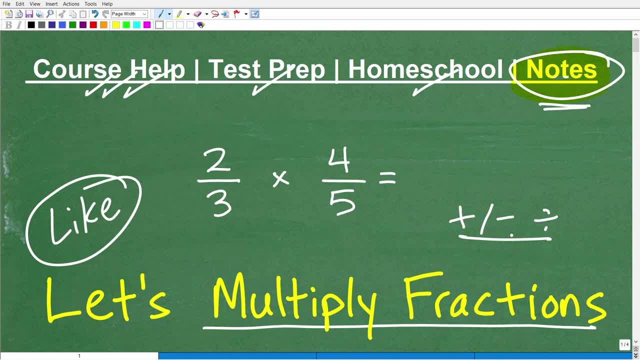 A Two courses. I would recommend a mine, one being pre algebra, which has a full chapter on fractions. but if you even want to go more basic than that, I have a foundations math foundations course that I go through, even basic arithmetic, basic addition, division, multiplication, numbers- much more basic- and fractions as well. so those are two additional options, but either way, please take advantage of my content that I post on YouTube if you like my teaching style. but my best math 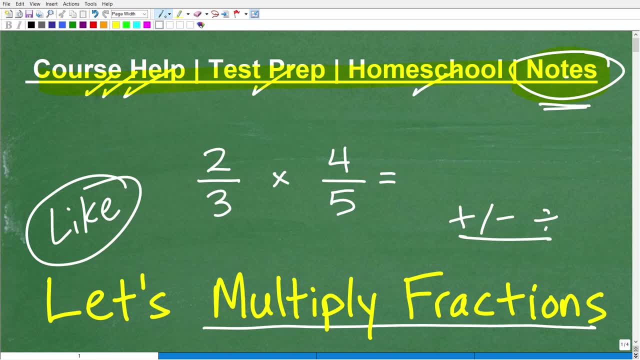 Help will always be within my math help program. okay, so, with that being said, I definitely wish you all the best in your mathematics adventures. thank you for your time and have a great day.